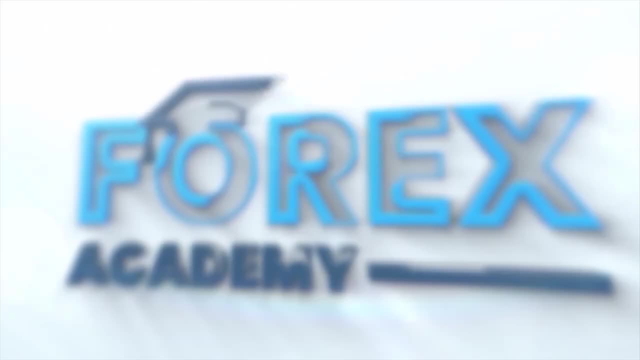 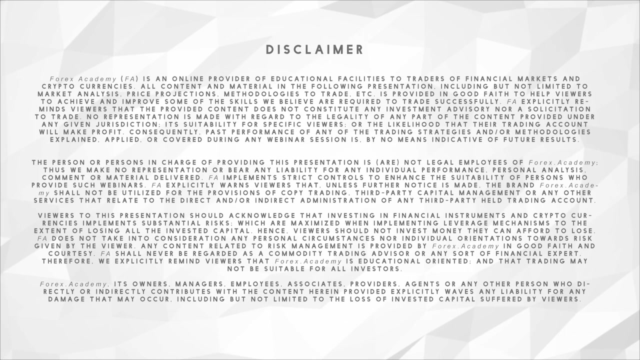 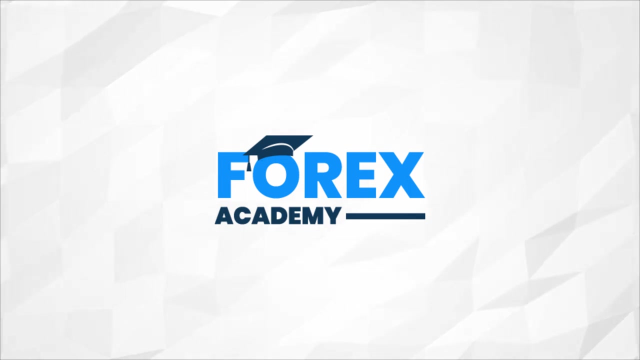 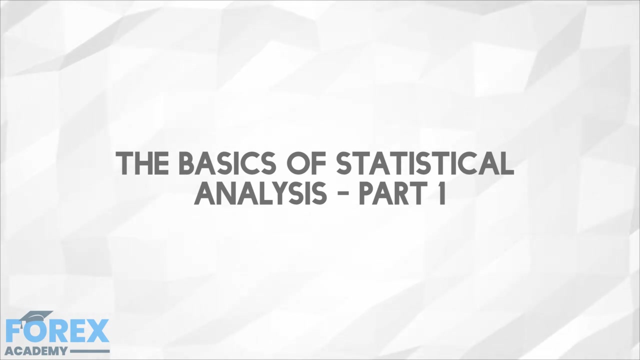 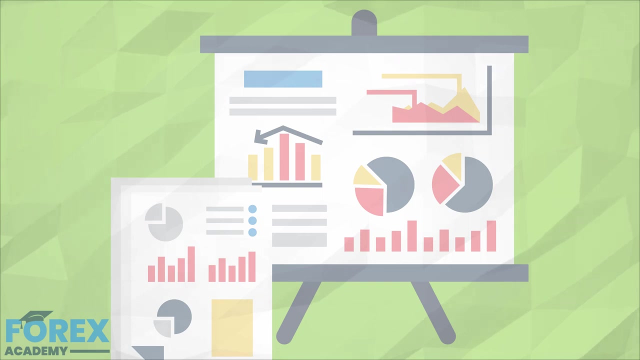 Hello and welcome to Forex Start Academy, your number one website for forex and crypto education and analysis. In today's edition, we're going to be looking at the basics of statistical analysis. Anyone interested in forex trading needs a basic knowledge of statistics and even basic rules governing probabilistic calculation. Do not worry about your ability. 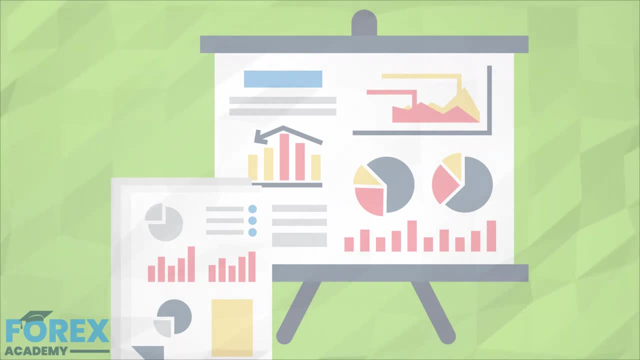 to understand this. we promise that you will, and it will be very simple and entertaining at the same time. Why do we need to understand this? A possible answer can be found in our latest video. why knowing your strategy parameters makes sense, but ultimately because, if you are serious about 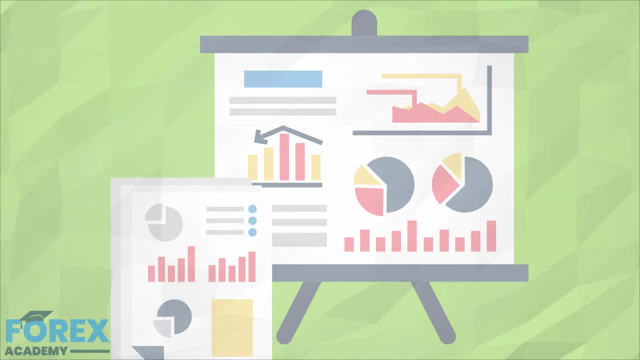 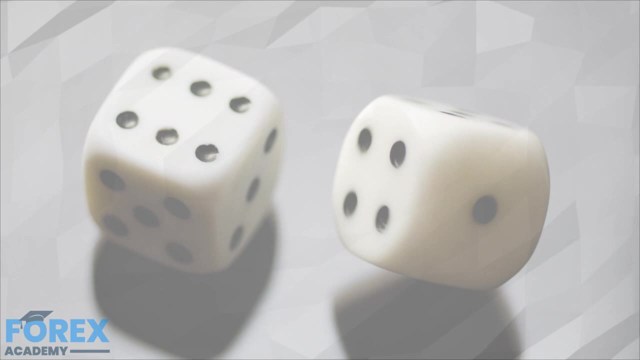 being a professional trader. this is one essential ability. you will need Basic terms. we need to know Probability. This area of math study involves predicting the likelihood of various outcomes, For instance, the possibility of your next trade is a winner. The mathematical area is a modern 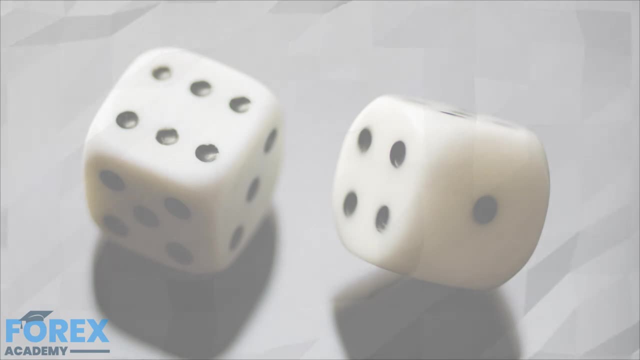 development of what, early on, was mathematics of gambling. Probability theory is also related to the theory of errors, of which Pierre-Simon Laplace was the first to propose, back in 1774, analytical formulas about the frequency of errors, Statistics. We can define statistics. 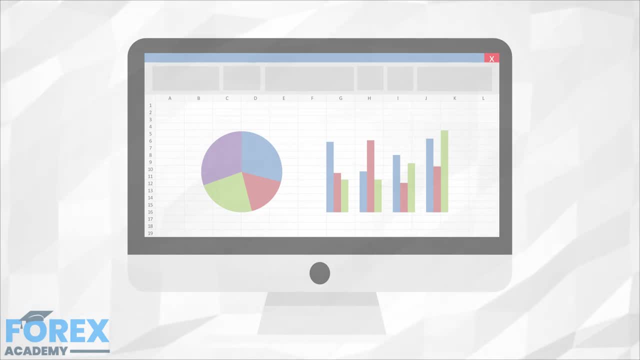 as a collection of facts belonging to a collection of events, objects or, more generally, a set. There are two kinds of statistics. Descriptive statistics try to describe a set in a useful way. We could, for instance, describe a typical Englishman by his average. 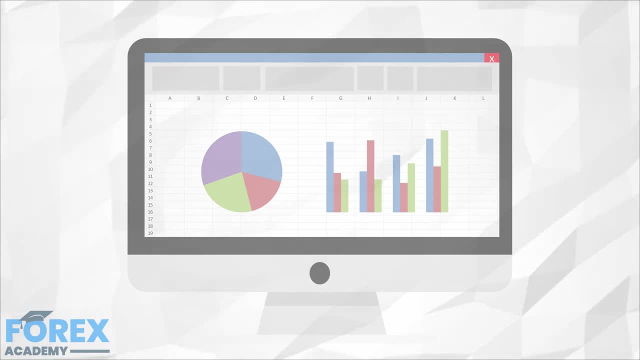 height, weight, number of hours sleep, the average income, the average number of males, and so on. Another type of statistics is inferential statistics or statistical inference. Sometimes it is not practical or impossible to measure all items produced by a process such as us on trading. 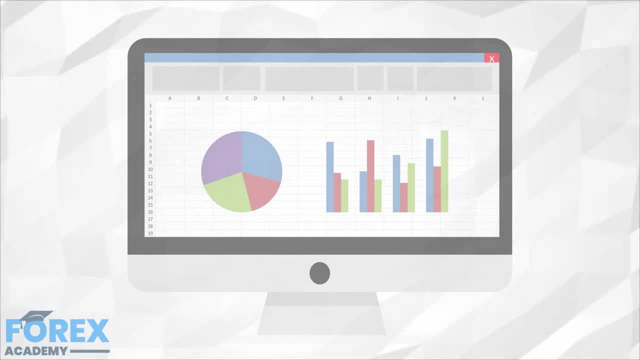 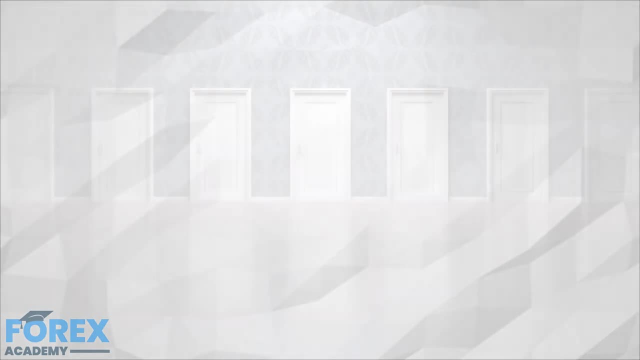 Therefore, we take a sample of the whole data collection and through it try to infer general properties or forecast its future events. We refer to chance if we know the event is uncertain to occur. Chance: We refer to chance if we know the event is uncertain to occur, Of course, if we see. 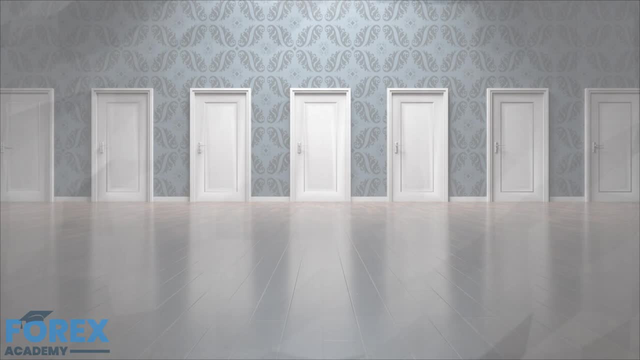 the event will always happen, for instance, like the sunrise. the chance is 100% sure. In trading, we use it in connection with the probability of a trade being a winner or a loser. Generally, we refer to the chance of an occurrence when we lack the specific knowledge for an event.